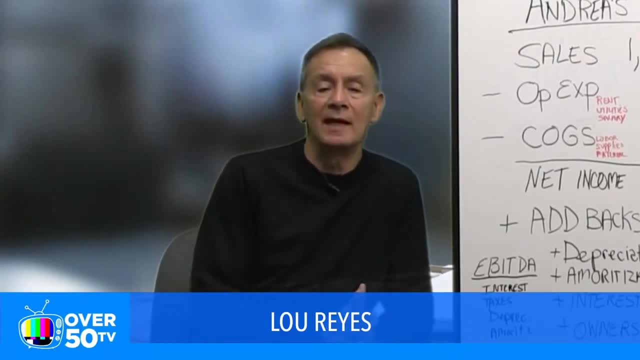 Years ago I was involved in the sale of a business that I started, and that was way back before the miracle of YouTube, when anybody could go on to the to the channel and find some video on how to to value a business. But again, I didn't have that luxury back then. so what I did is I went out like 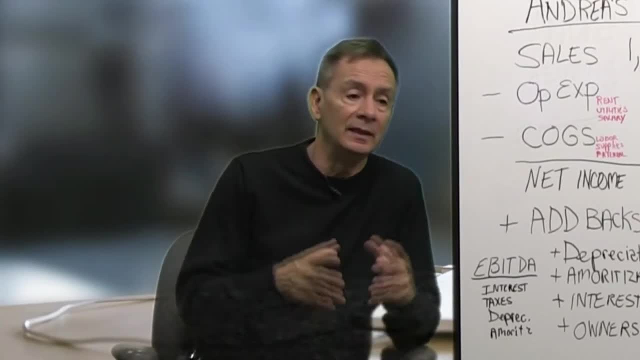 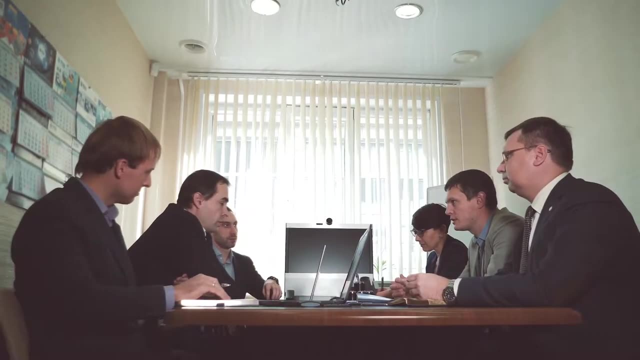 a lot of people did, and I went out and got myself a business attorney, talked to him, asked him to represent me. We went into the negotiation and I remember sitting there and it was a kind of an intense negotiation and I remember sitting there thinking you know what? this isn't going the way I 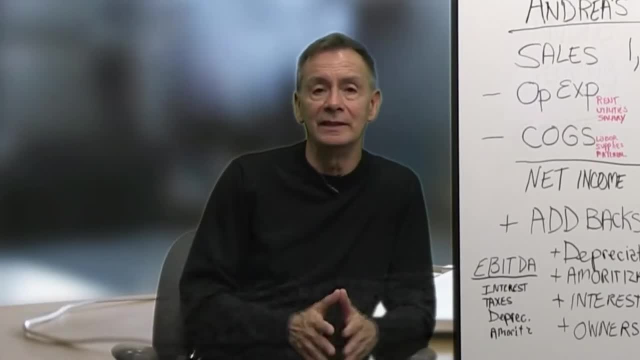 wanted to, But I leaned on the knowledge of the attorney. I believed that what he was telling me was correct. We went ahead and finally, after some intense negotiation, we finally arrived at a price. and bam lo and behold, I walked out of that meeting and I thought: you know, this just isn't right. This 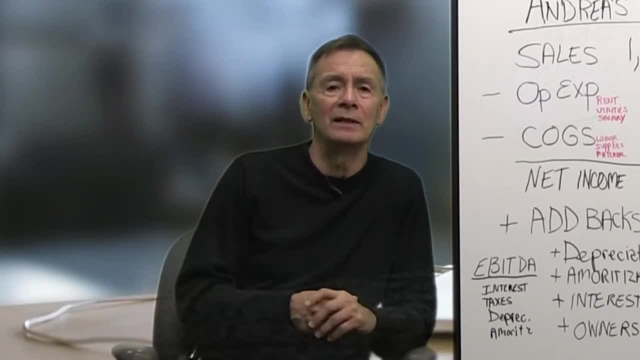 number. it's not right. But you know what I'm going to go with, what the attorney's recommending. and and here, soon afterwards, I realized I found out that I sold that business for less than its real value. And you know what I did to myself? I promised I would never let that happen again. So what I did is since that. 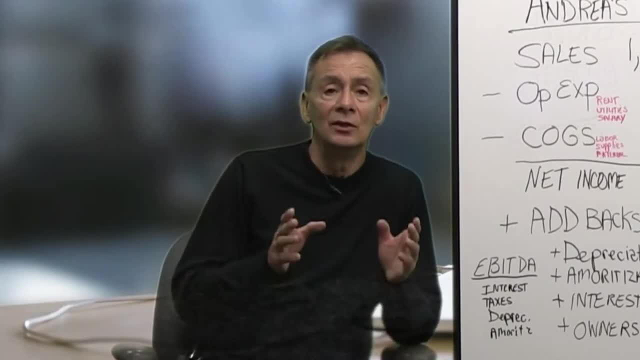 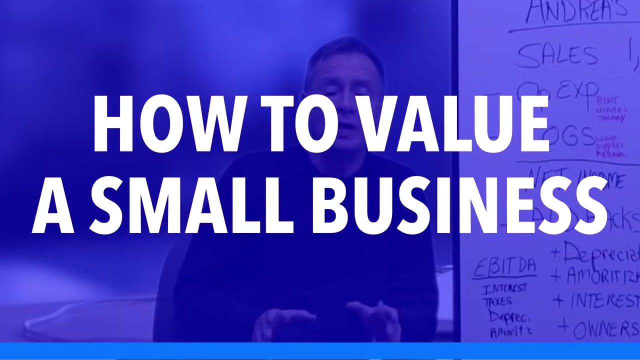 time. I have spent quite a lot of hours learning how to price a business, learning how to value a business, learning how to do negotiation in a way that was going to benefit me and was going to benefit my family. So what I want to do now is share with you how to value a small business. 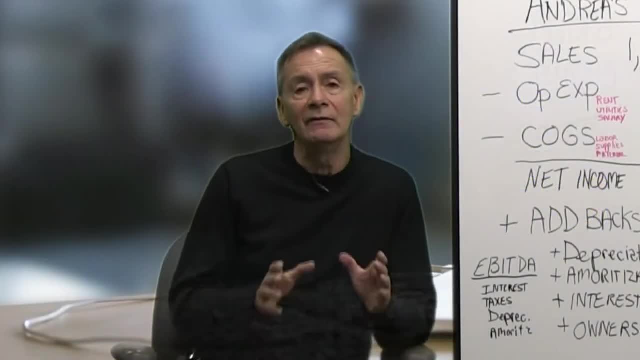 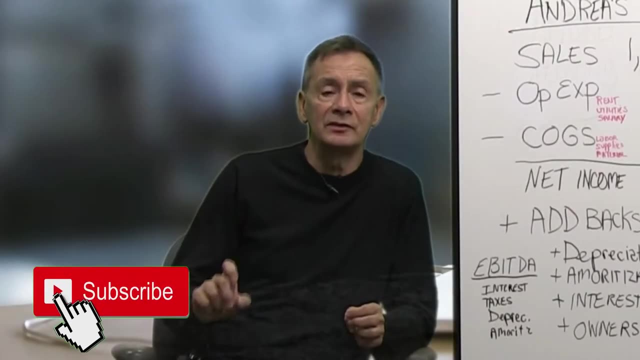 But before I do that, I want to remind you that if you haven't already subscribed to our channel, please go ahead and do that. All you've got to do. there's a little button underneath the screen and if you click on that button that says subscribe, you'll go ahead and you'll subscribe our channel, but there's a little bell next to it. If you click on that, 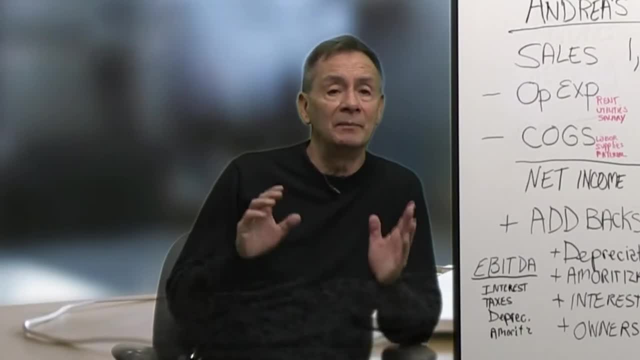 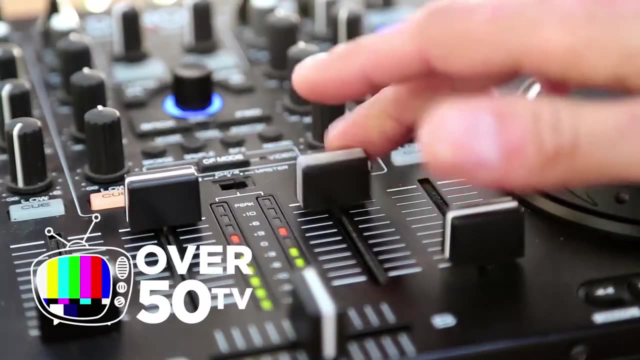 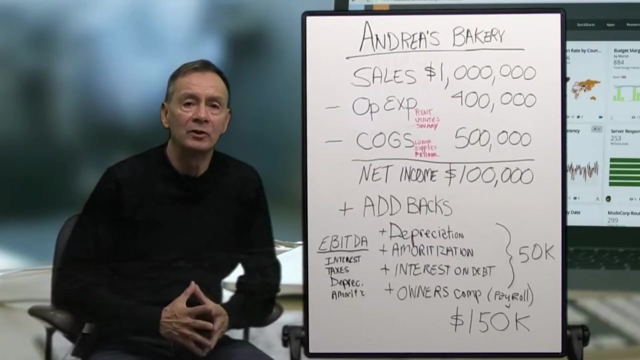 little bell. you'll get the latest updates. They'll be delivered right to your inbox. So, without further ado, I'm going to go ahead and have Scotty tune it up. Welcome back to Over 50 TV. and what I did here is I have an example that I put on this: 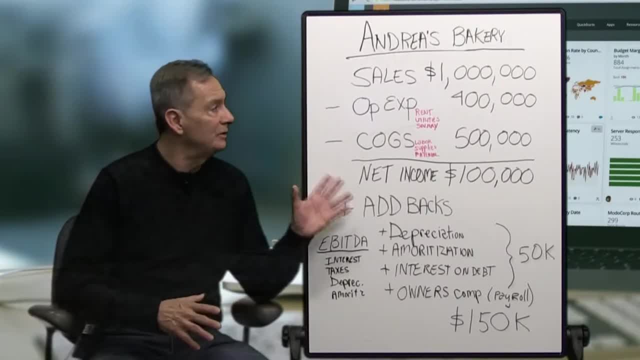 whiteboard. I have an example of a business and I thought I'd do this just basically as an illustration, to give you an idea on pricing and how to price a business. But before I go through this board here, what I want to tell you is I'm going to do this. 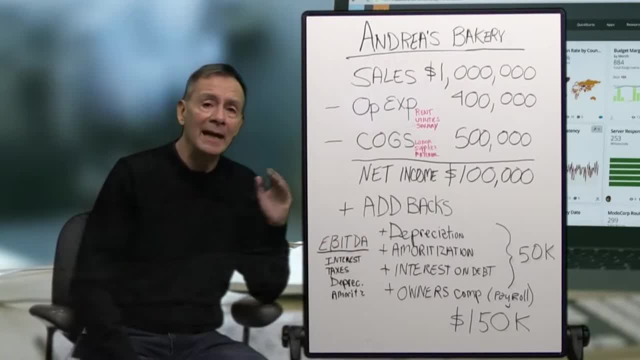 in two parts. Number one is I am going to give you this example, But then, after I do this, after I go through this example, what I want to do is go over some key facts, things that I know that you should know before you sit down with anyone. 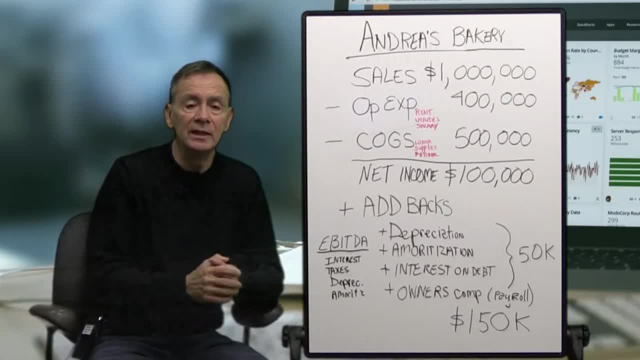 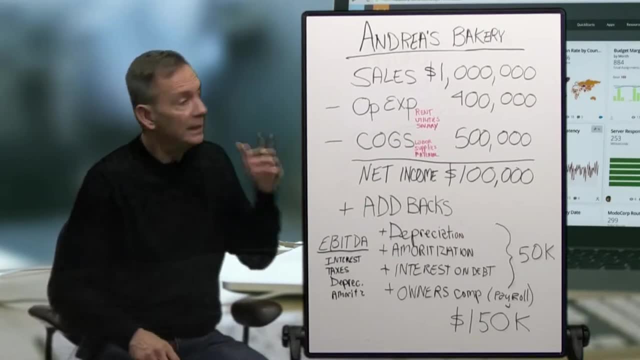 to do a pricing or a negotiation, But really to get the true value of a business. you're going to want to look at part one and part two, So let's go ahead with part one here. And what I did is I put together here a business. 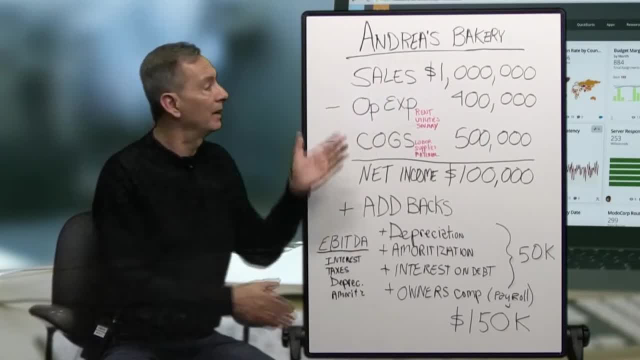 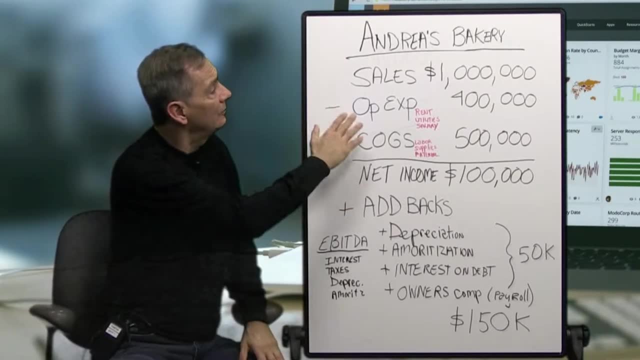 Now there's an Andrea's Bakery. I don't know any Andrea's Bakery, but I did this just as again, just to illustrate. I wanted to give you an idea on some pricing. So let's go ahead and look at this. 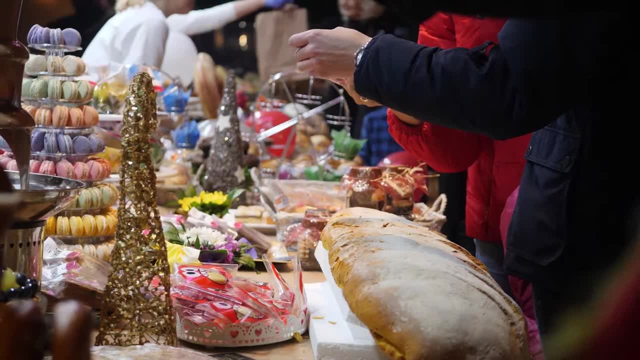 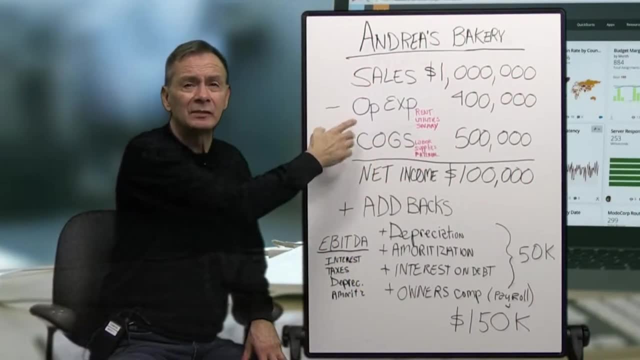 Andrea's Bakery does a million dollars a year in sales. Now for a million dollars she has operating expenses And operating expenses. this is right off. If you look at a tax return, you're going to see this information right on a tax return. 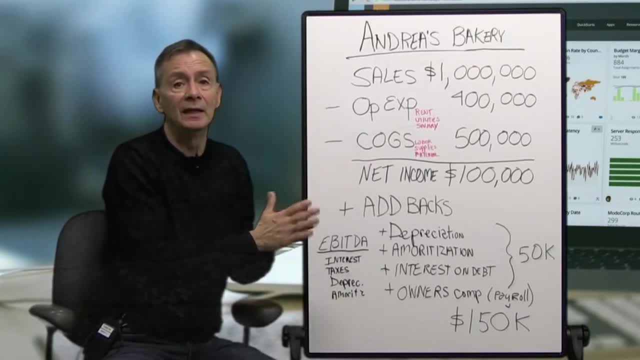 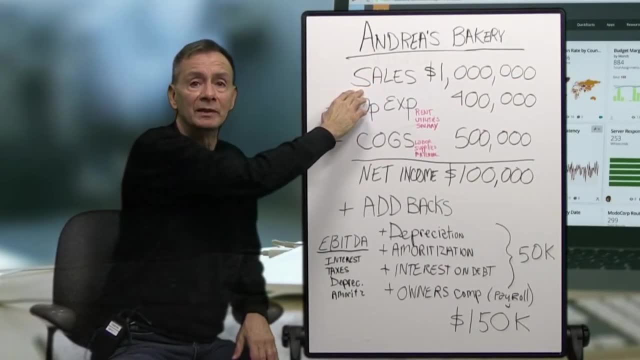 But really it's basic information that it should be on just about any income statement. So you've got here Andrea's Bakery. She's got sales of a million dollars per year. She has operating expenses of $400,000.. And operating expenses, really what that is is that includes things like rent. 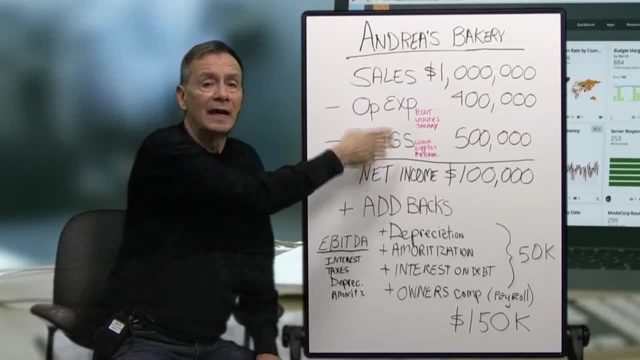 That includes utilities And that would include the salary for Andrea if she was taking out a salary. And I imagine in this example, here, yeah, We're going to say she's taking out a salary, But here, yeah, She's taking out a salary- 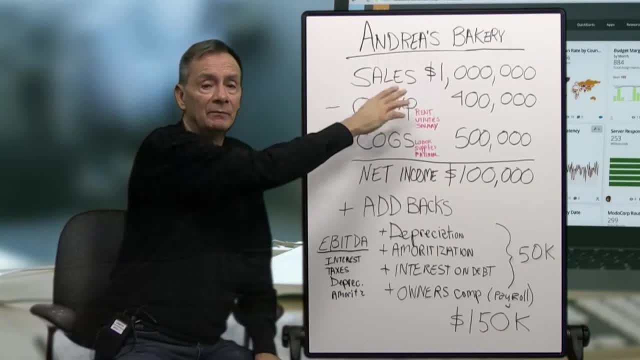 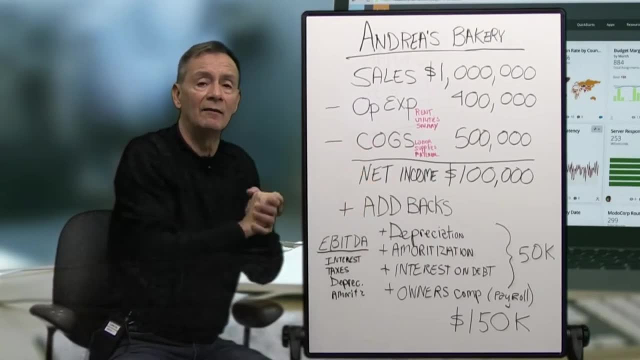 Now from that again you subtract the $400,000 from the million And then you've got what we call the cost of goods sold. And in the cost of goods sold that's the cost of the product, the cost of making the 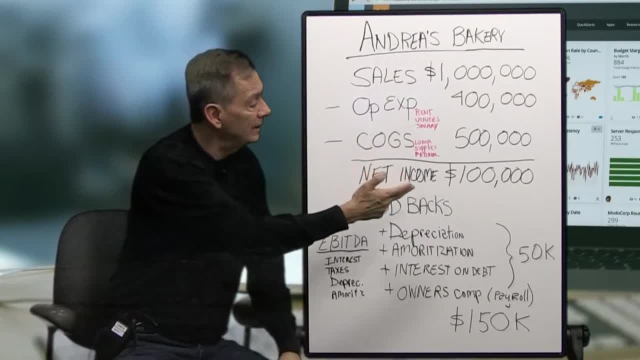 product, And that would include labor- what you're paying somebody to help you or paying a few people to help you. In this case, with a million dollars in sales, I would imagine she's got a few employees- Supplies, And it also includes things like material. 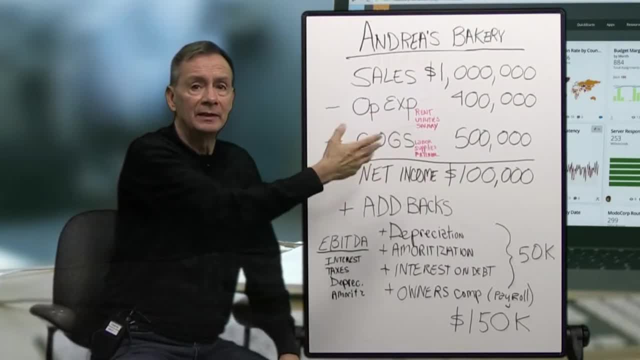 But you can go ahead again. in income statement you can see more, or even on the tax return you can see what kind of items are that they have that are listed on that statement there. But you've got sales of a million. 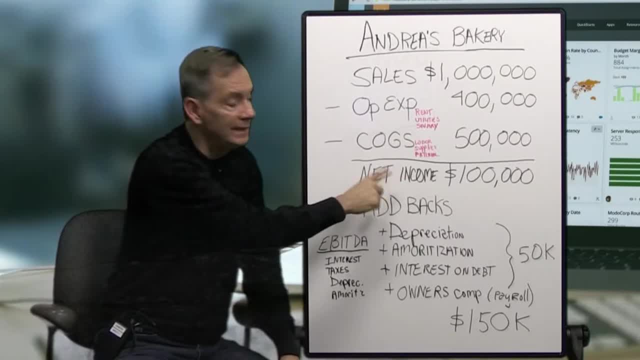 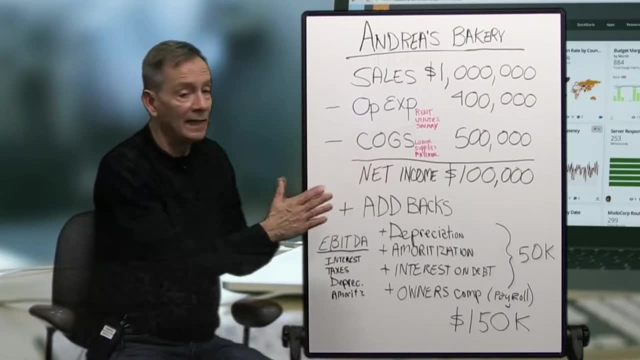 You subtract the $900,000. Her profit, her net income. let's say her net income is $100,000.. Now some people would look at that and say, and I've worked with people, I've actually worked with people who say, Lou, you know, my business is worth a million. 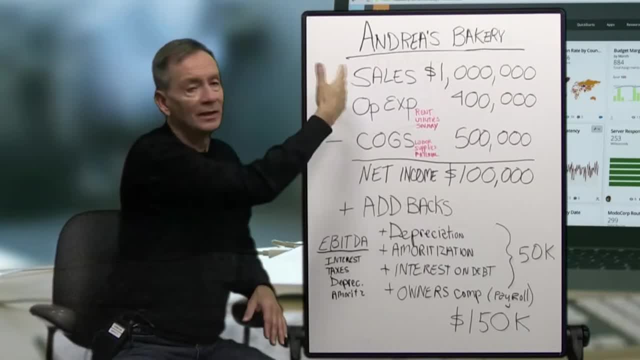 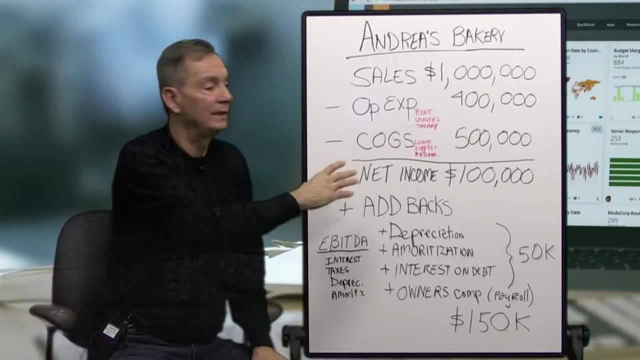 And then I'm going to do a multiple of that. So I'm going to sell it. It's really worth $2 or $3 million And I'm always letting them know. no, that's not how you value a business. You really want to get down cash flow. 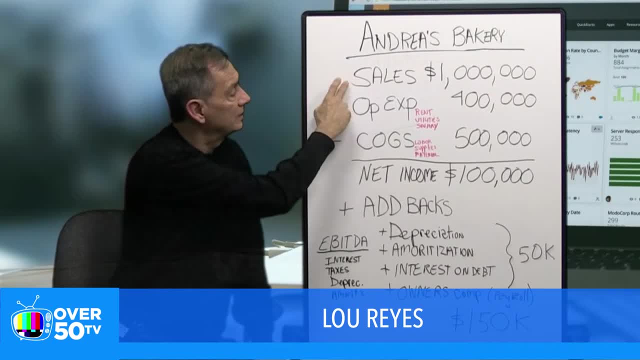 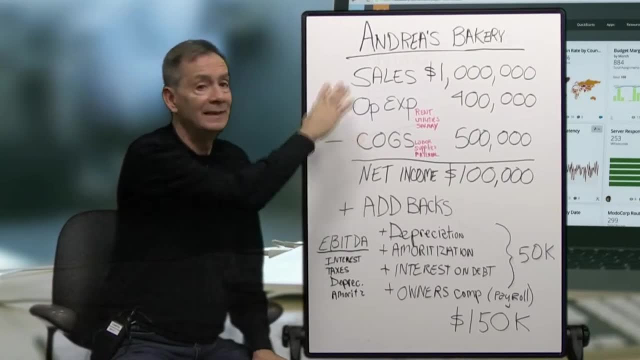 You want to get down to net income, And that's what we've done here. So sales minus operating expenses, minus cost of goods sold is going to give you your net income of $100,000 in this example. Now there is something else that's called add-backs, and I listed that here. 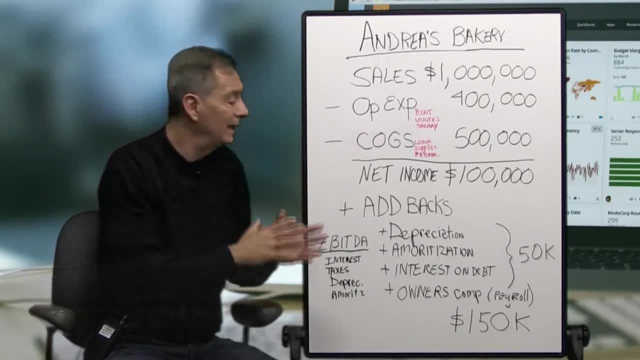 And these are just a few of the add-backs, And what I'll do is I'll go ahead and I will tell you some of the other add-backs that you can use or you should be aware of when you're looking at valuing a business. 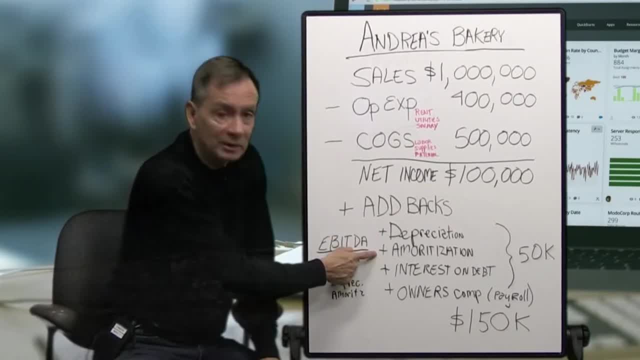 But in this case I've listed depreciation, amortization and I've listed interest on debt, And then I've got the owner's compensation through payroll, when they're paid through payroll, And that would be right back into the operating expenses. But again you've got the net of $100,000.. 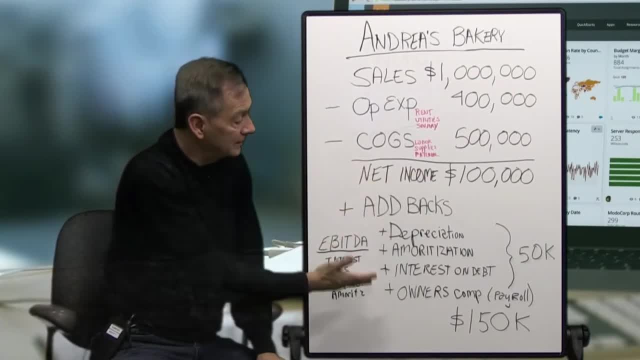 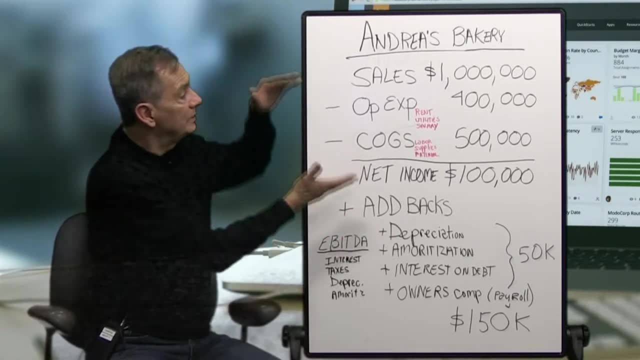 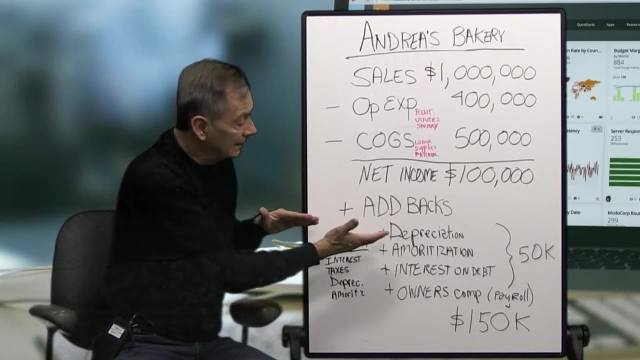 You're going to add back to that amount And I put about $50,000, and these are arbitrary numbers. Again, this is an example here for you. But you're taking your sales minus your expenses, You're adding back to that some key categories and again I've got them down here. 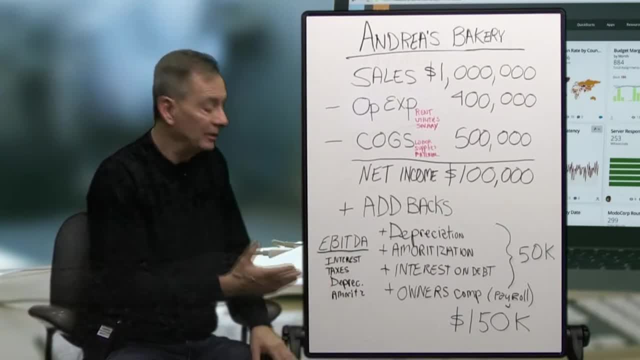 And what's called really in financial parlance- and you've probably heard it- it's called EBITDA. EBITDA- I'm trying to say that properly, But EBITDA is interest. It's interest is taxes, depreciation and amortization. 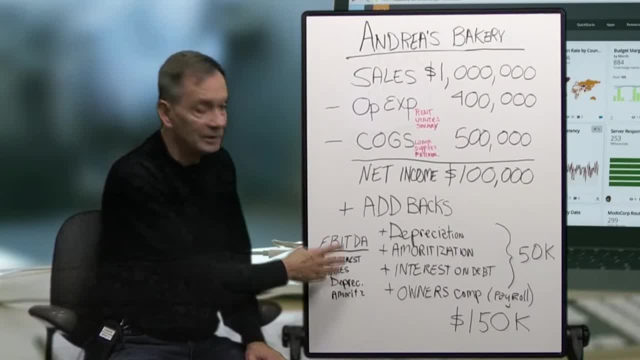 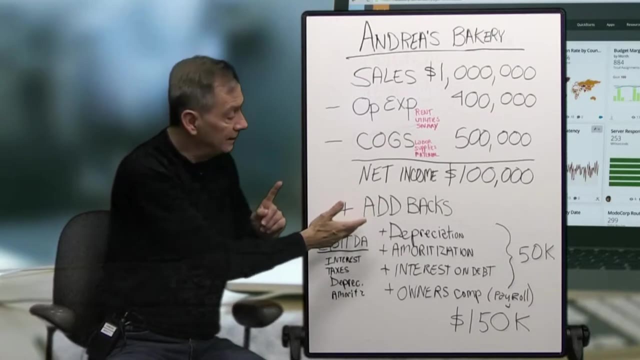 So it's earnings before these four items. So that is what your EBITDA is, So you're adding back these items. Now let me say this to you though: okay, So we're coming up with a value of the business, and this is a value based on sales for one. 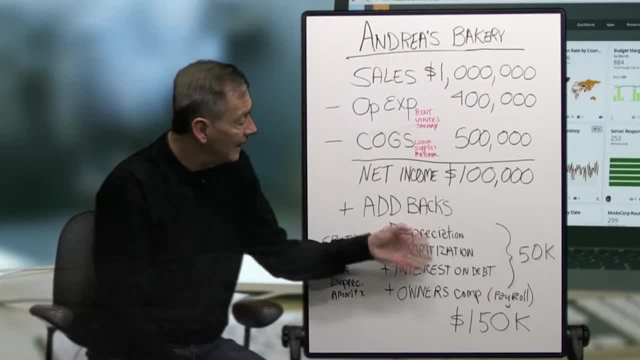 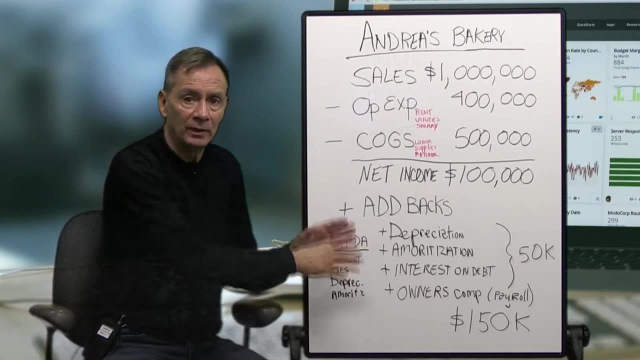 year. It's based on adding back expenses. So if you add this amount back, that business could be worth $100,000.. Okay, That business could be worth $150,000 without the multiple, and this is what we're going to be getting to in the second part here. 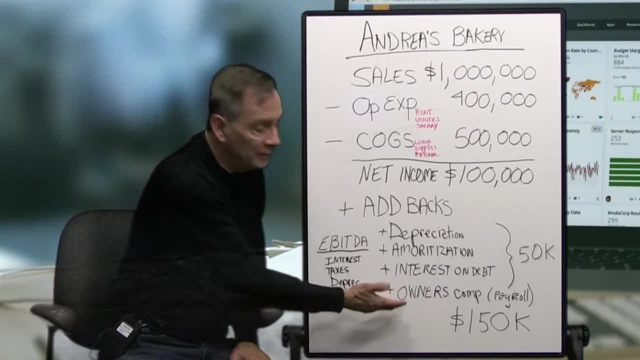 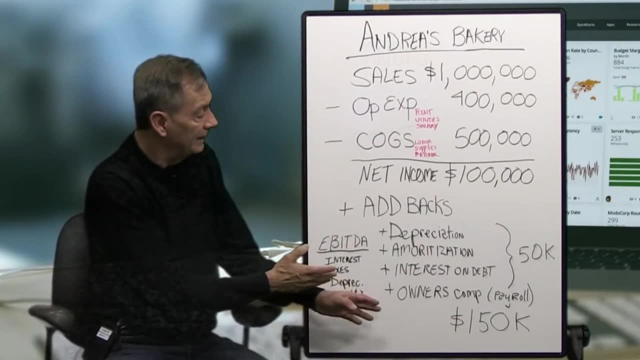 But again, I'm looking at this for one year of a value, for one year of $150,000.. Now, when you're looking at this amount here, you're saying, okay, wait a minute. You know, at least I've learned over time. I've learned that there are going to be other. 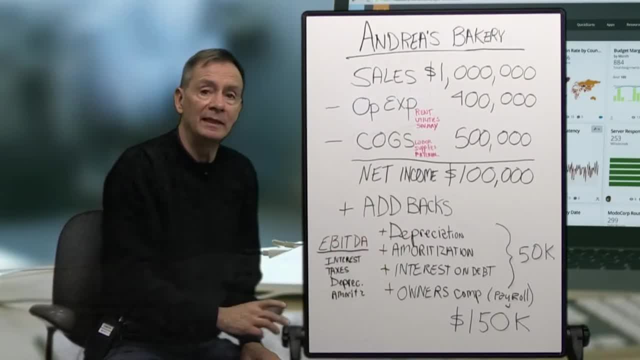 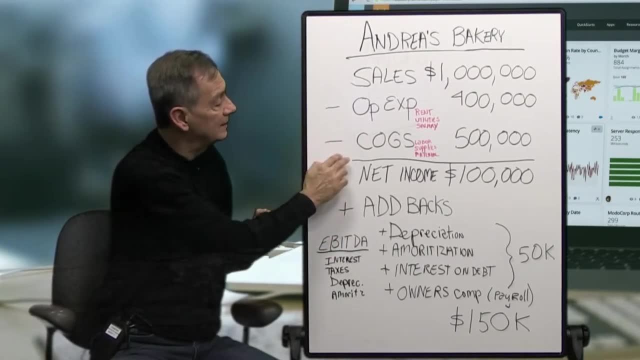 add-backs. There's things that aren't listed in here, And let me give you an example. Many business owners- Business owners- will put expenses or bury expenses into operating expenses. They might even do something into cost of goods sold, But what they'll do is they'll put in here. an example would be entertainment expense. 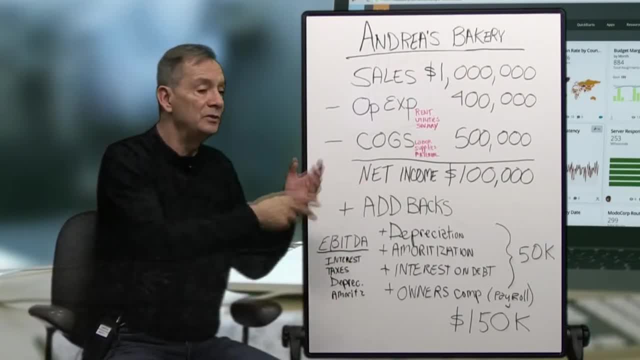 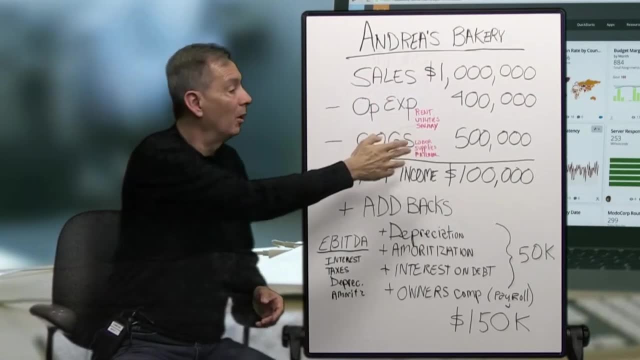 Say they bought a boat and in that boat they're using that for entertainment expenses. So they're going to subtract what they pay for that boat on a monthly basis or however they decide to do that, But they're going to put subtract or add into that operating expenses. 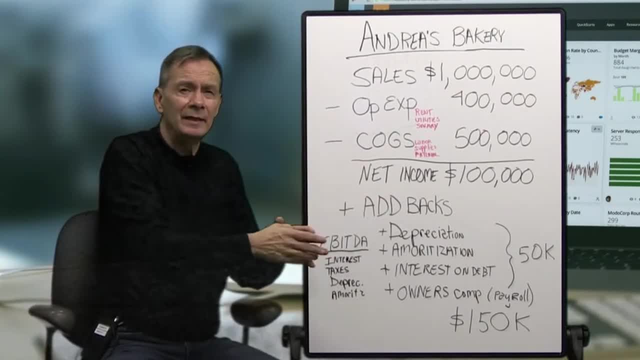 They're going to add in what they're paying for the boat. They could have a huge monthly insurance bill because they Health insurance bill because they have a particular illness. that means that their insurance premium is going to be higher, So that could be also added in here. 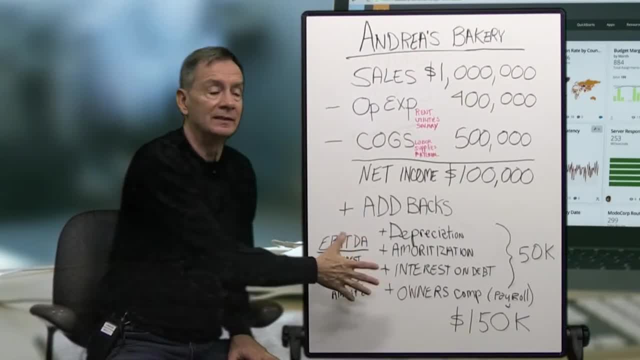 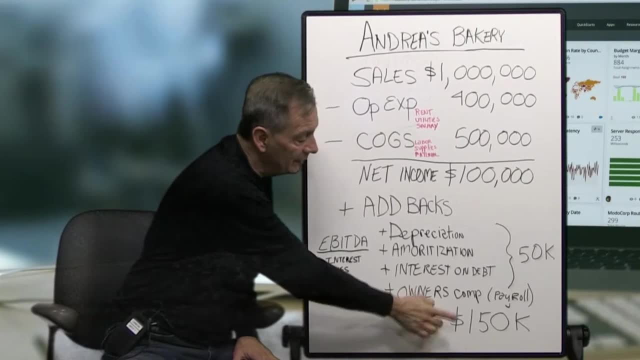 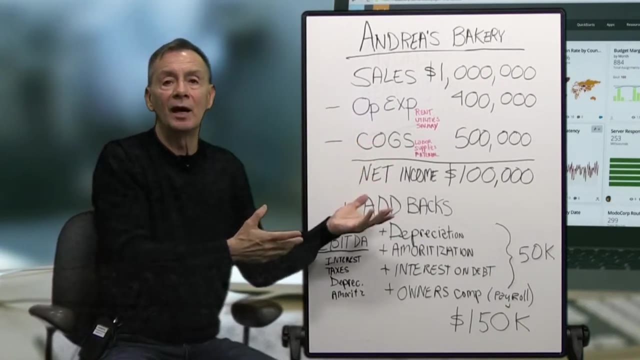 So there are add-backs that are in addition to this that you've got to be aware of, And when you have those add-backs, when you subtract them And you add them to here, that number could go up significantly Again. it could be a boat, it could be health insurance, it could be multiple cars. 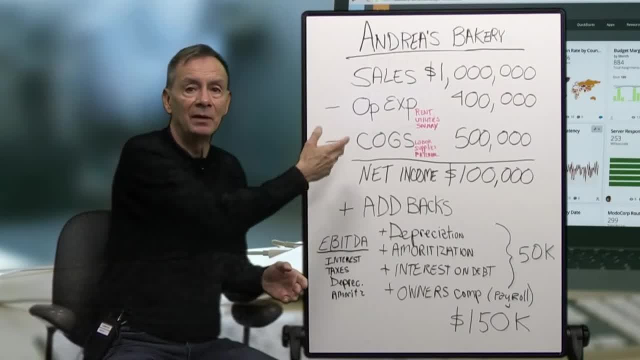 Maybe they put their wife's car in here or their husband's car a monthly payment in here. Those add-backs always should be. You should scrutinize the statement. I recommend you look at the income statement But more importantly I look at the tax return. 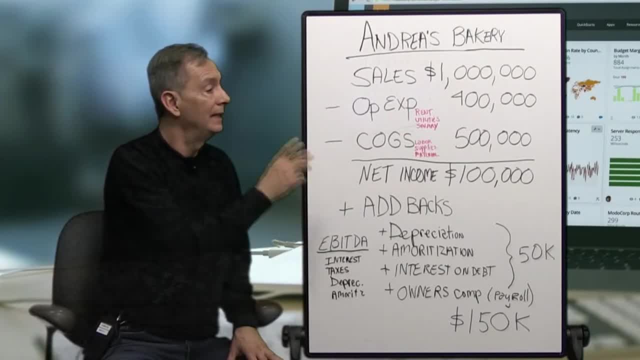 Because if I'm valuing a business, I'm looking at that tax return And I'm seeing What they put in there, What they have in their operating expenses and what they have in their cost of goods sold, Because I'm going to be able to. 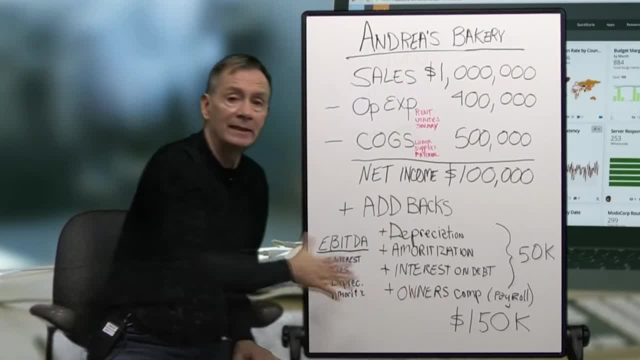 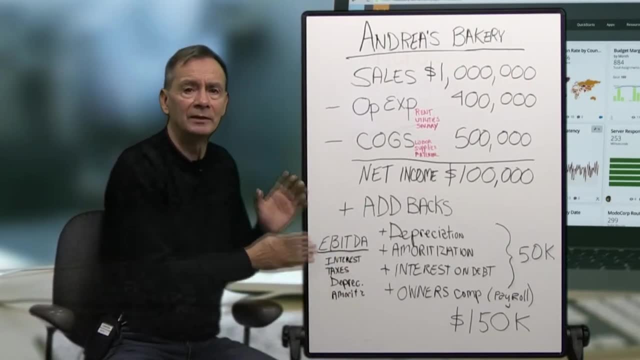 I'm going to want to pull those numbers out and add them down here so I come up with the true value of the business. So this is basically just a quick summary. I want to get you in the ballpark to understand what you're looking at. 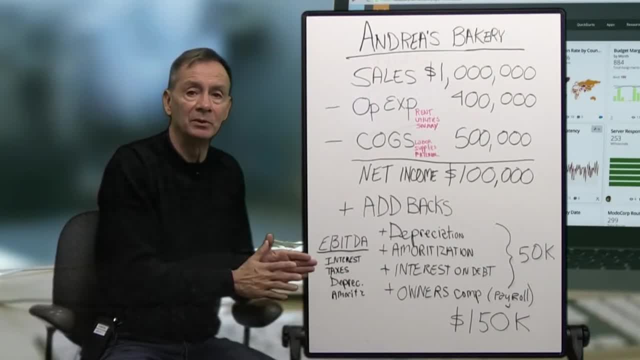 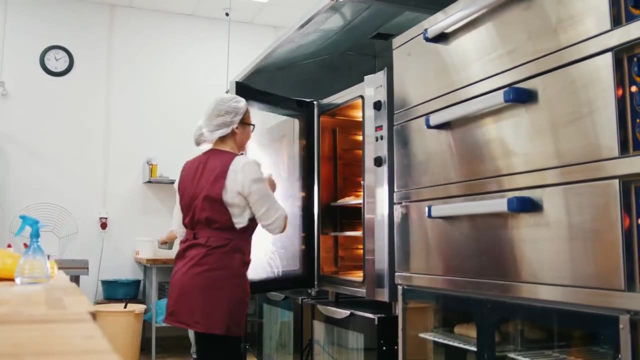 Now, what I want to do now is: I'm going to be talking about multiples And I'm going to talk about things like risk, because those are also factors whenever you're coming up with a price for a business. Okay, we're going to talk about some other things here. 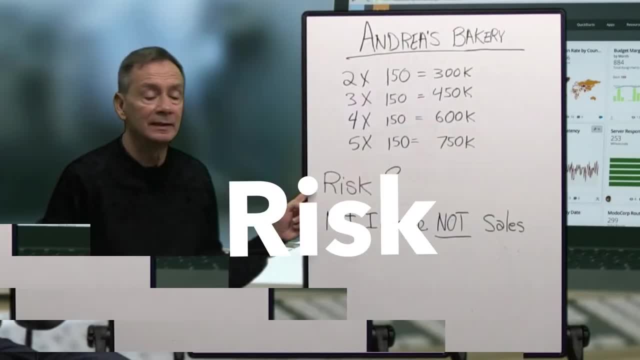 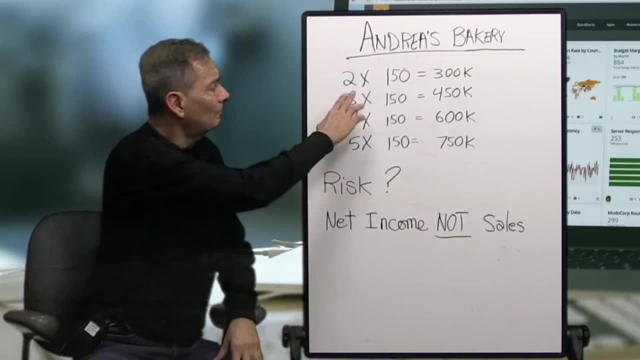 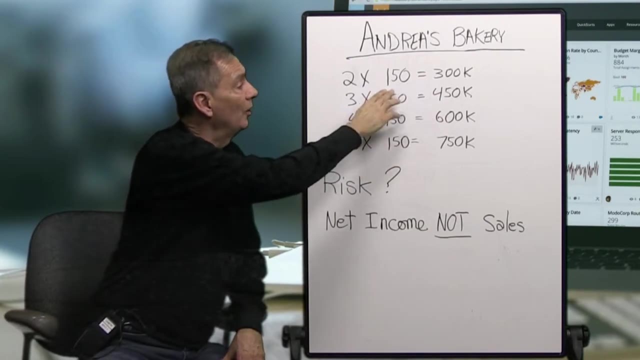 And we're going to talk about multiples and we're going to talk about risk, And then I want to stress to you that we're really talking net income, We're not talking sales. So here's where we go. We said that Andrea's Bakery was worth, at least on an annualized basis. she had $150,000.00.. 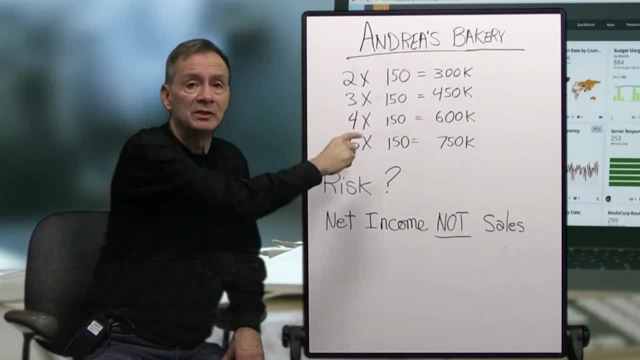 Wow, $150,000.00 in value for that business for the year. And what I'm saying to you is this: that there are something called multiples. So you could take that $150,000.00 and you could say her business is worth a multiple. of two, so that business would be worth $300,000.00.. If you took a multiple of three, the business is worth $450,000.00.. Four multiples $600,000.00.. A five multiple is $750,000.00. 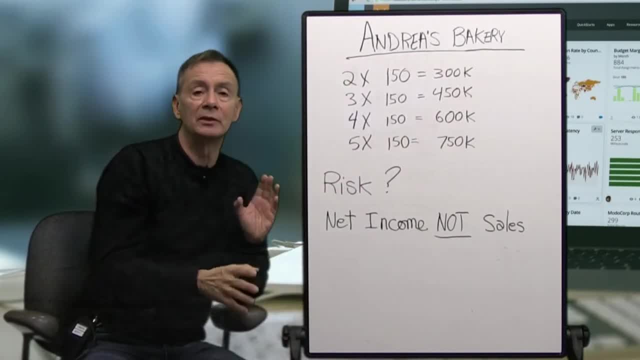 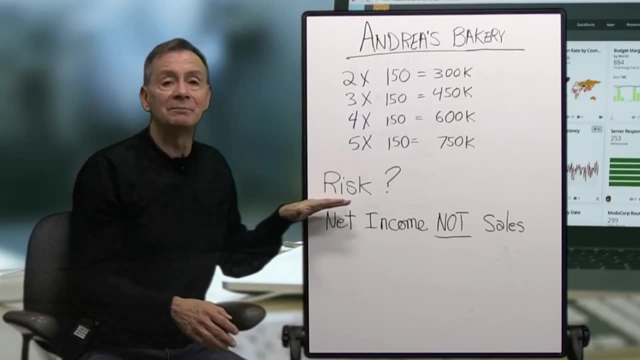 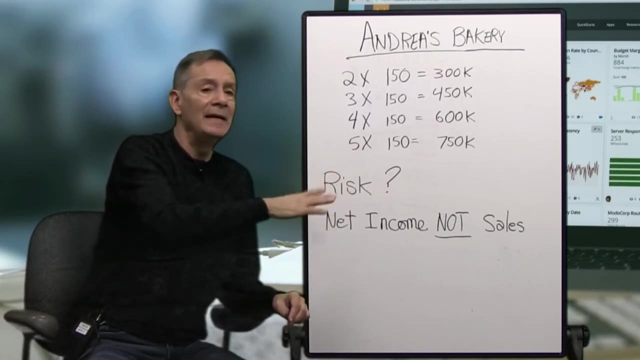 Usually on a small business. what I find is your multiples are going to be around two to three, So you get a two or a three time multiple Multiple. really, it's based on risk. If you have a small business and you're doing under a million dollars in sales, you may. 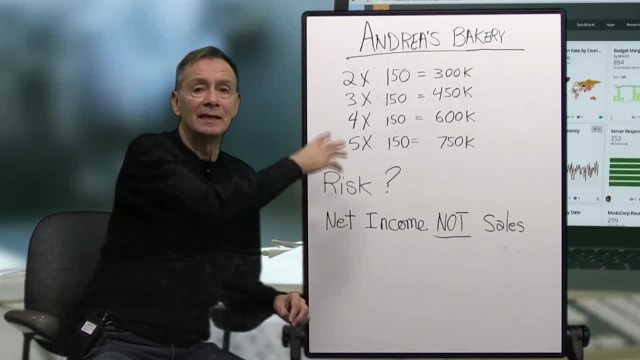 have a little bit more risk than if you have a business that's doing more than a million dollars. And I'm going to say that and that's not something that's going to be etched in stone, obviously. The reason I'm saying that is because a business that's doing a million dollars in sales usually 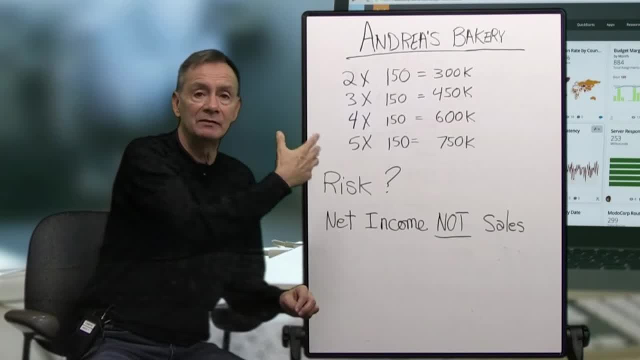 or more than a million. usually you have some support system, You have some employees, You have a little bit of a machine who's generating that kind of a revenue. So that's when I talk about risk and maybe a little bit lower risk and a higher multiple. 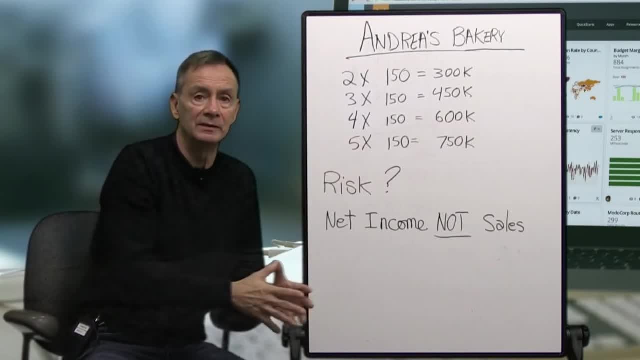 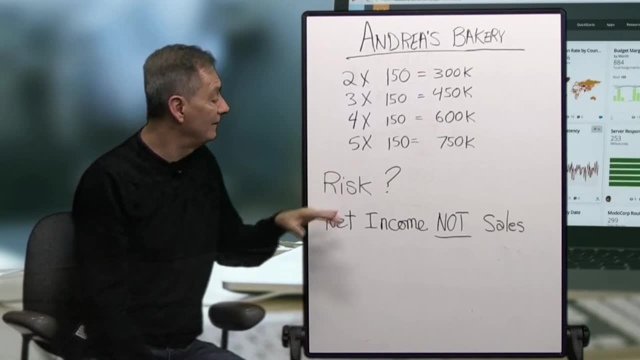 is because you have more of a machine. more longevity in the business is what I'm also going to assume, And I'm making some assumptions here. but again, you've got multiples: two, three, four or five. It's all based on risk. 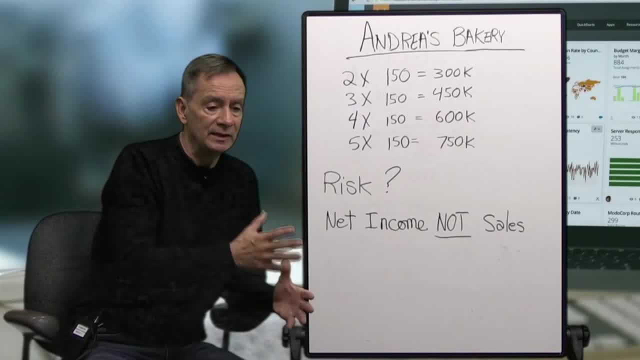 You know, I told you in the beginning of this video that when I was sitting down negotiating the sales of a business, I remember the person I was negotiating with said to me: he says: well, you know, we don't know if this business is going to be around in a year or two. 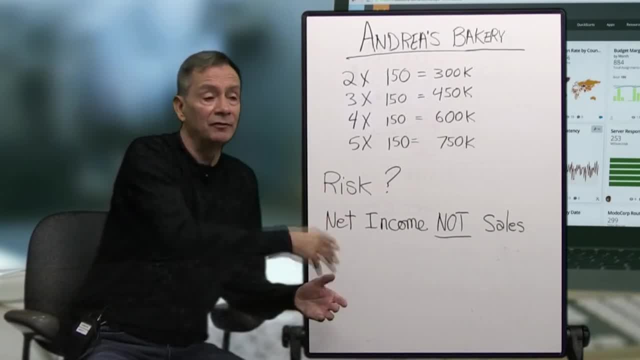 And I said, well, yeah, but the business has had steady growth for the last few years, And I don't mean small little incremental growth of, you know, three to 5%, I'm talking 15 to 20% growth in that business. 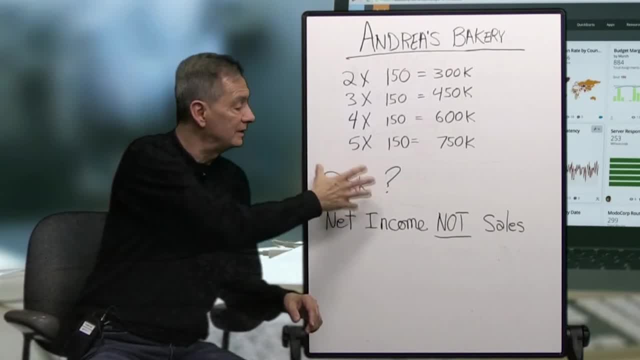 So he went ahead and really looked at risk and use that as a way to try to get the value of the business down. But multiples depending, they all depend on risk and that's what you want to look at. So, if you are talking about buying a business, if you're looking at selling your business, 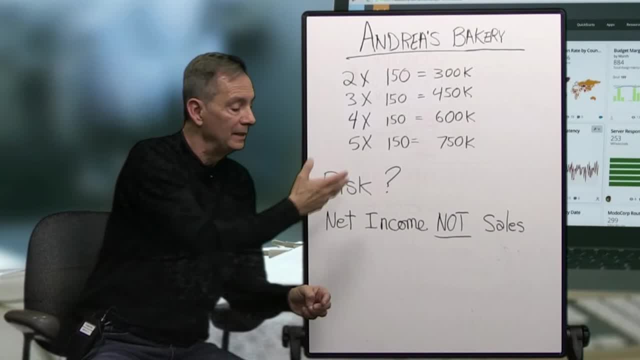 you want to consider the expenses that I listed, the sales and the expenses I listed in the first part of this video, But then again, after that, you're looking at multiples. All I'm trying to do here is just get you in the ballpark. 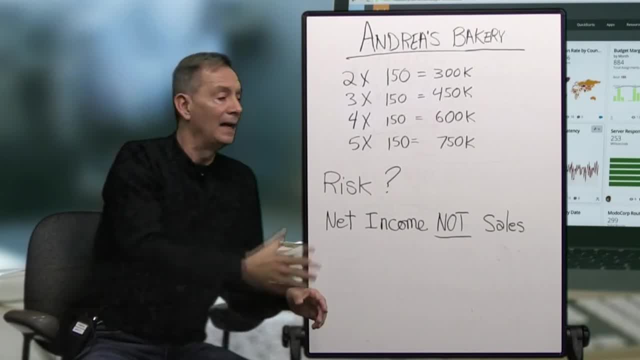 You know if you're looking to sell a business or buy a business. I want you to understand these, like you understand the back of your hand, But I also recommend that you find someone who you can talk to, someone who has experience in buying and selling businesses. 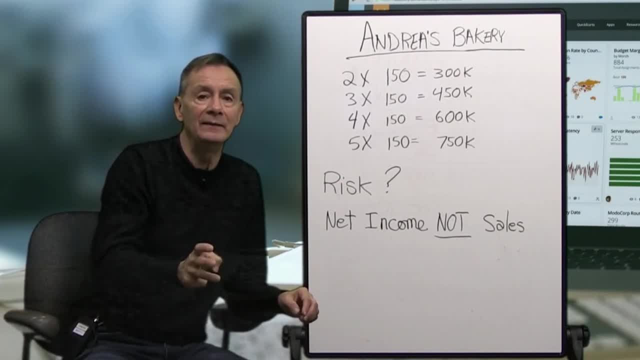 Talk to them. It's going to be worth the investment. It'll be worth what you pay them. It's going to be worth it because they're going to help you to get the true value of your business. So that's about all. 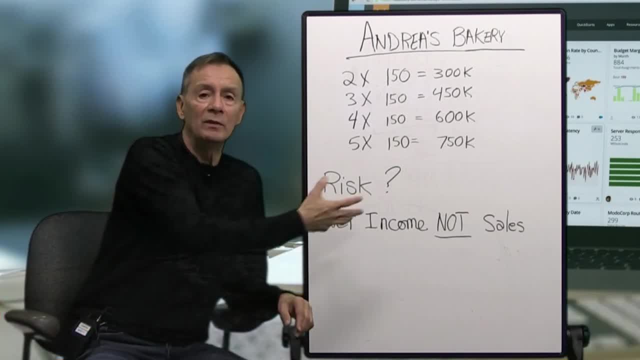 That's about all I've got for you for today. If you have any questions, you can always make comments in the comments section here on our YouTube channel, But for now I want to thank you for watching the video And, again, if you haven't subscribed to our channel, please go ahead and do that. 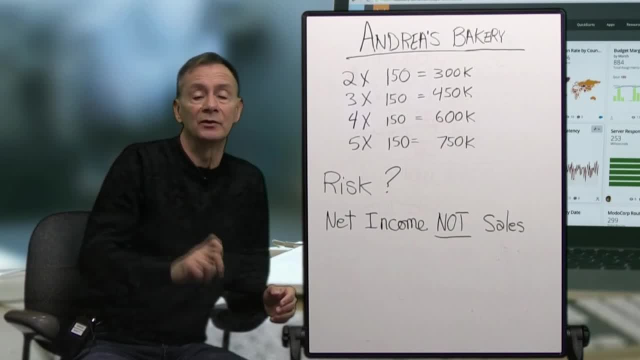 All you got to do is hit that little subscribe button And also, if you hit that little bell, you'll get our latest updates. So this is Lou Reyes with over 50 TV. I hope I've helped you and I hope you have a great day everybody. Bye, Bye, Bye. 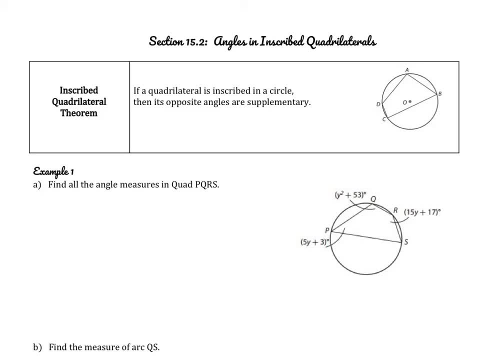 Hi everyone, this is Mrs Gia, and today we're going to talk about angles in inscribed quadrilaterals. So here you have an image of an inscribed quadrilateral in a circle. So notice that all four of your corners are on the circle and your quadrilateral is entirely within the circle.